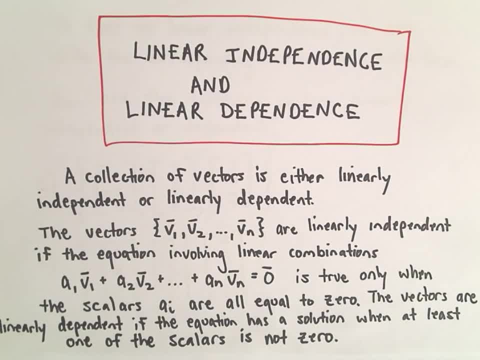 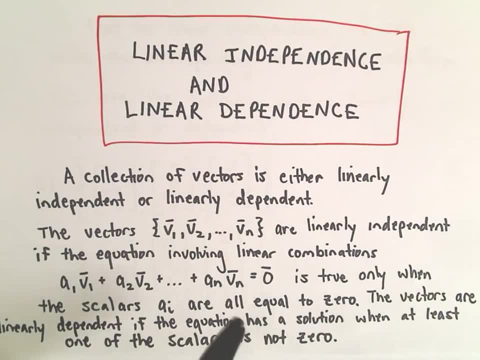 All right, in this video I want to look at the notion of linear independence and linear dependence. So a collection of vectors is either linear independent or linearly dependent, And what we say? so we say, the vectors v sub 1, v sub 2, v sub n are linearly independent. 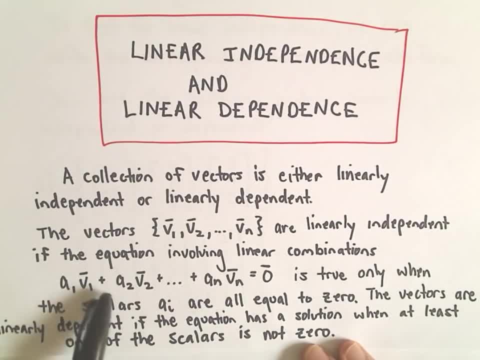 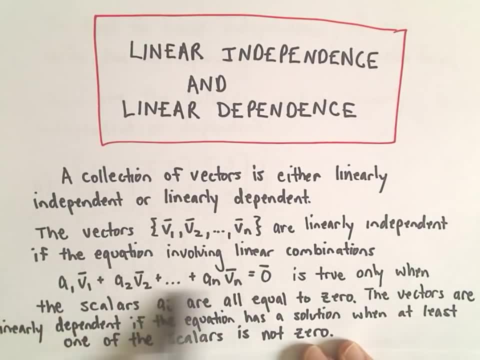 If we look at the linear combination, a sub 1, v sub 1, plus a sub 2, v sub 2, plus dot, dot dot up to a sub n, v sub n, when we set that equal to the zero vector, if the only solution to this equation 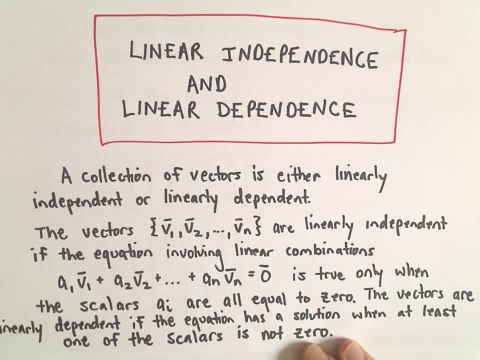 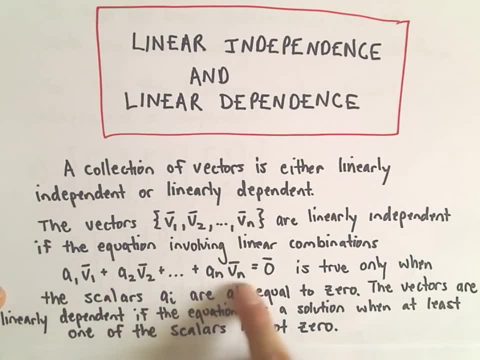 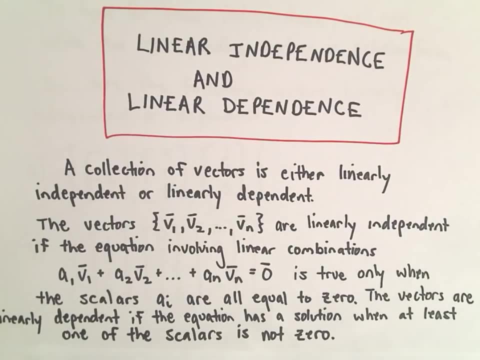 is when the a sub 1, a sub 2, a sub n are all zero, we say those vectors are linearly independent. If this equation is true when at least one of the a sub i's is not zero, well then we say at that point that the collection is linearly dependent. 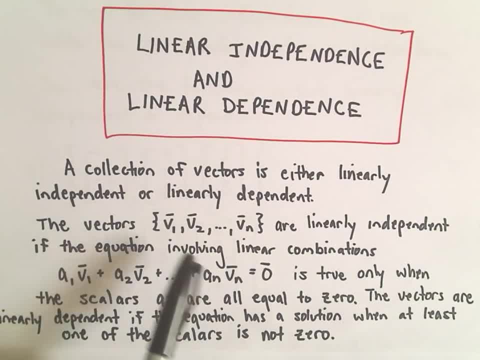 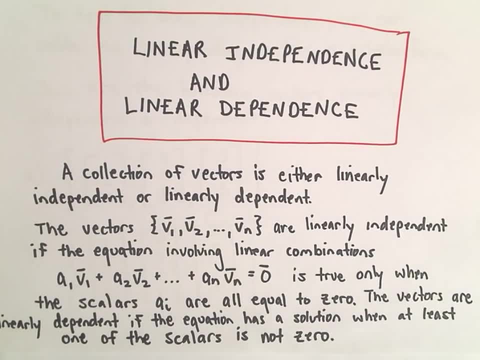 And kind of intuitively I guess, the notion: if you have a collection of vectors that's linearly dependent, in a sense you kind of have some redundant vectors in the sense that you have a collection of vectors that's linearly dependent. So if you have a collection of vectors that's linearly dependent, 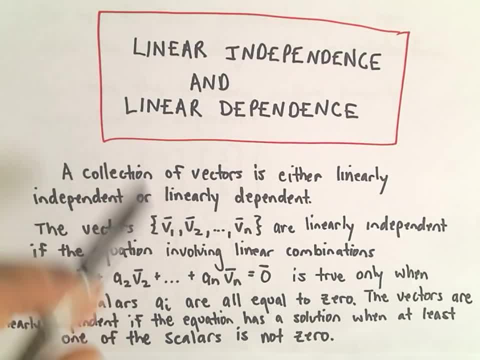 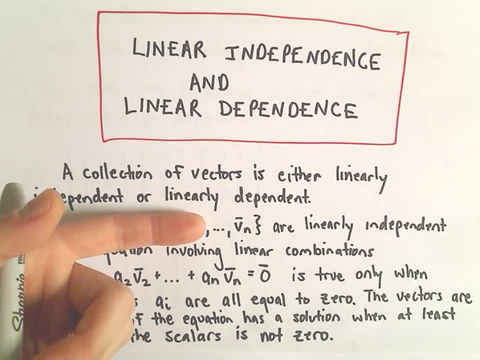 you can get rid of some vectors if it's linearly dependent, you know. chop it down so that you only have, you know, fewer than what you started with, And the idea is you can still write any vector in that space as a collection of that smaller set of vectors. 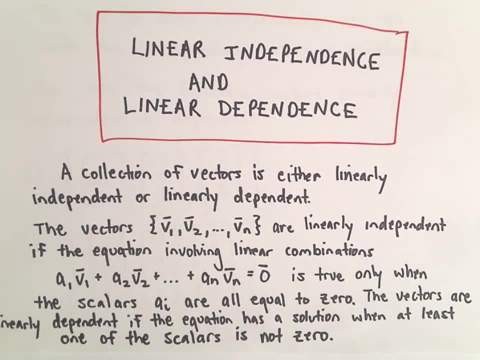 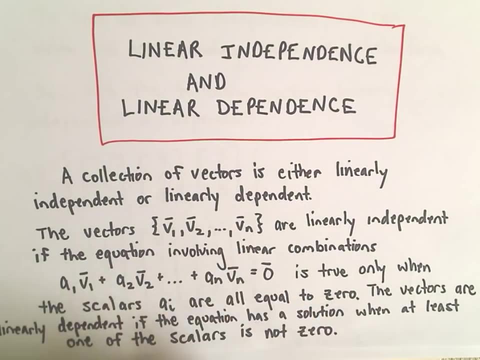 That's the notion of linear dependence You kind of have. you basically have vectors that are linear combinations of the others and therefore in a sense they're not needed. So we're trying to chop down our set, make it as small as possible so that we just sort of have the fewest number of vectors. 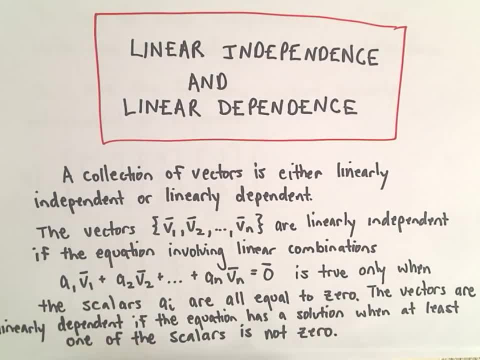 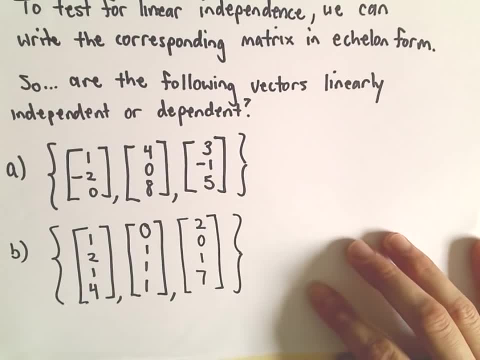 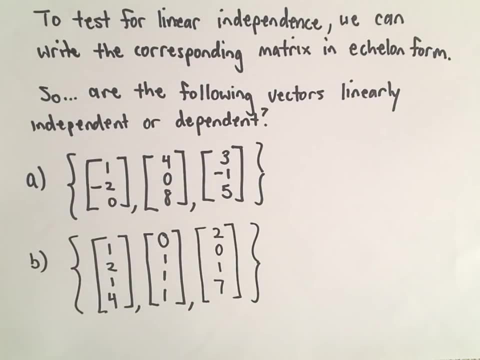 so that we can write any vector in that space as a combination of those remaining ones. I guess it's kind of that to me is the intuitive idea. If you have a linearly dependent set, somehow you got too many. If you have a linearly independent set, well, hopefully you can use those to not necessarily write the other vectors. 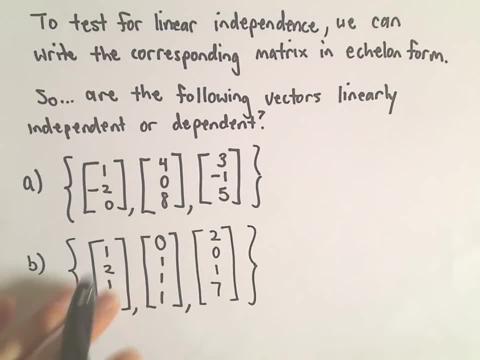 all the other vectors, But ultimately you can write the other vectors, But ultimately that's what we're trying to do. We're going to try to find a small enough set so that we can write the other vectors in terms of those remaining vectors. 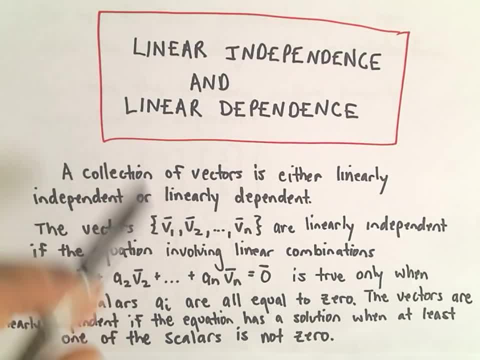 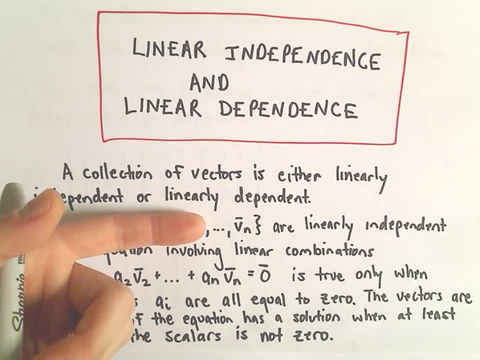 you can get rid of some vectors if it's linearly dependent, you know. chop it down so that you only have, you know, fewer than what you started with, And the idea is you can still write any vector in that space as a collection of that smaller set of vectors. 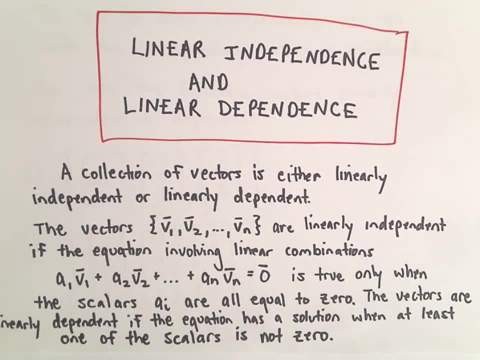 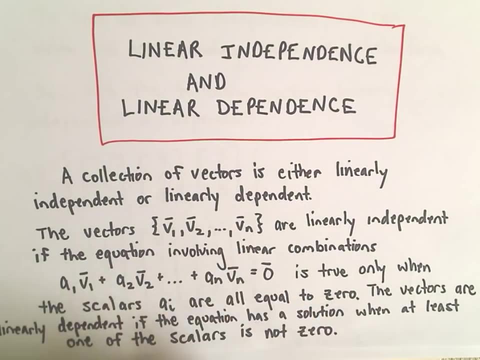 That's the notion of linear dependence You kind of have. you basically have vectors that are linear combinations of the others and therefore in a sense they're not needed. So we're trying to chop down our set, make it as small as possible so that we just sort of have the fewest number of vectors. 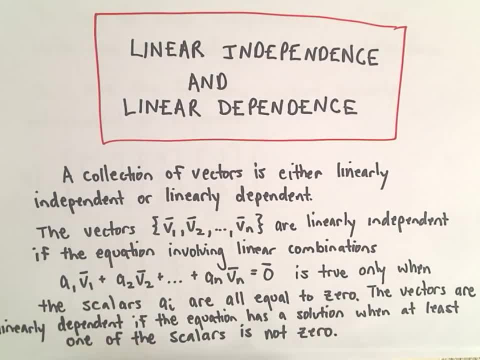 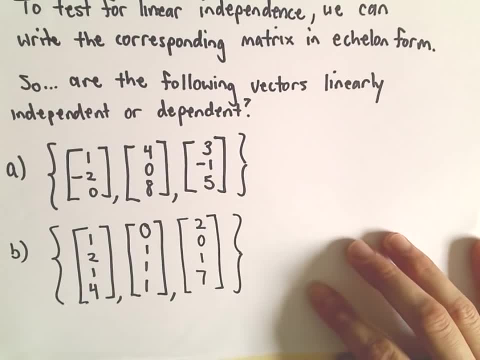 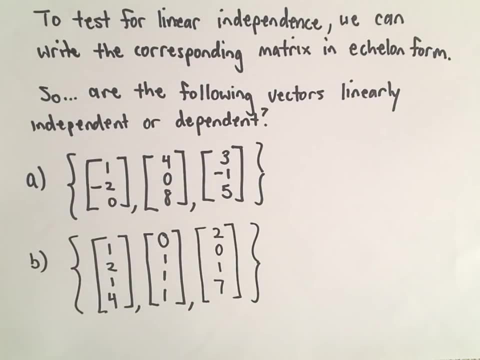 so that we can write any vector in that space as a combination of those remaining ones. I guess it's kind of that to me is the intuitive idea. If you have a linearly dependent set, somehow you got too many. If you have a linearly independent set, well, hopefully you can use those to not necessarily write the other vectors. 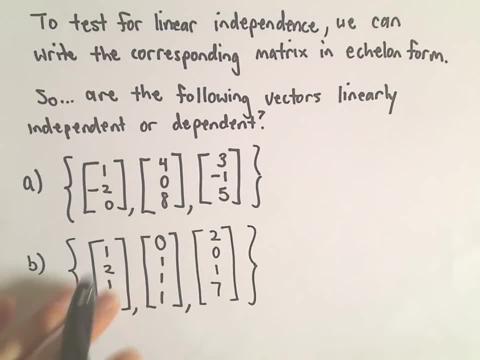 all the other vectors, But ultimately you can write the other vectors, But ultimately that's what we're trying to do. We're going to try to find a small enough set so that we can write the other vectors in terms of those remaining vectors. 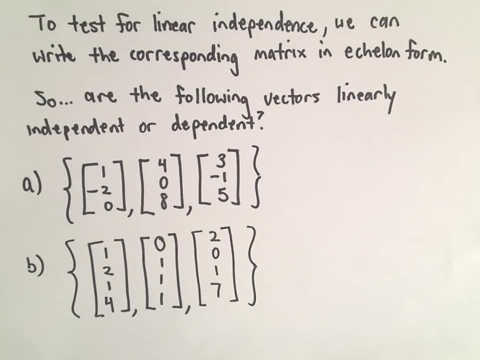 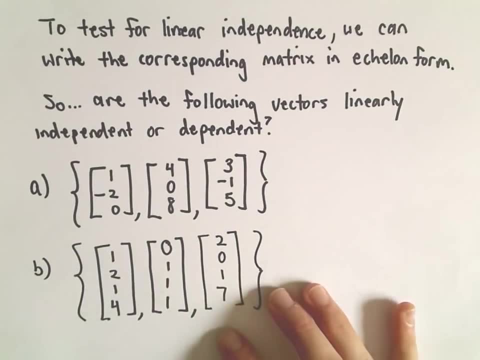 And this is what ties into the notion of the basis for a vector space. But again, we're not there yet. So again, just at this point, think intuitively. Somehow, if you have linearly dependent vectors, those are just linear combinations of other ones. 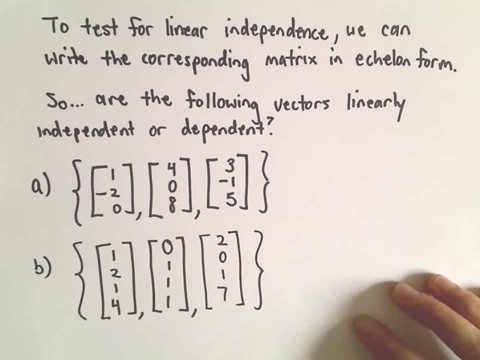 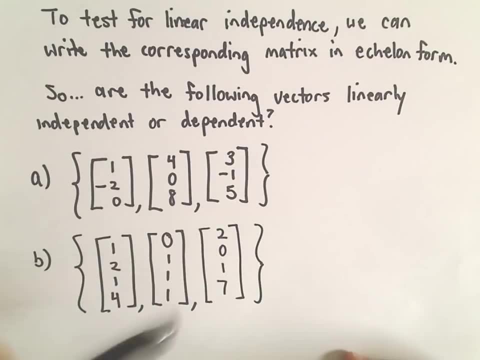 So, in a sense, you can get rid of them and you're not losing any information. That's how I think about it. Okay, so just two questions here. We've got two sets of vectors, two different examples. We'll do these in two different videos. 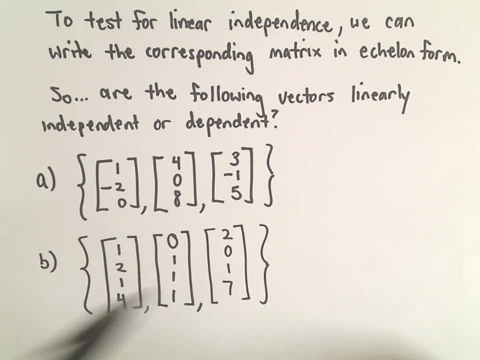 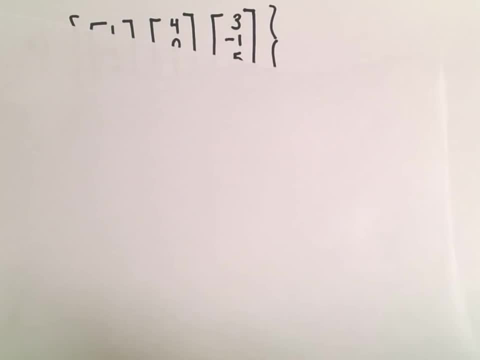 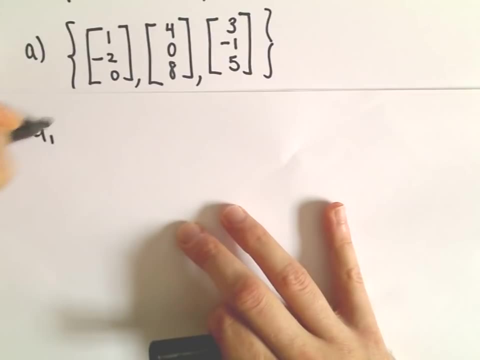 And we're just going to decide if these collection of vectors are linearly independent or dependent. So we'll do part A here first. So again, what we're doing is we're just looking for solutions to the system of equations, or the equation a sub 1 times 2.. 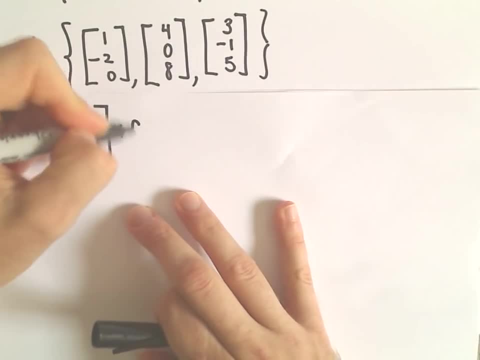 And again, if we were to do that with a vector, that's just the same as A sub 3. we would just divide that by 2.. And again we have A sub 3, A minus 2, 0. So what we have here is A sub 2 plus A sub 3 times 1, negative 2, 0 plus A sub 2 times 4, 0, 8.. 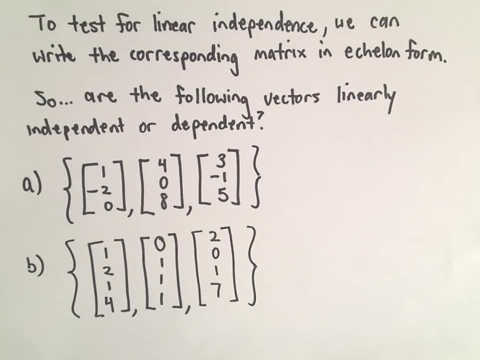 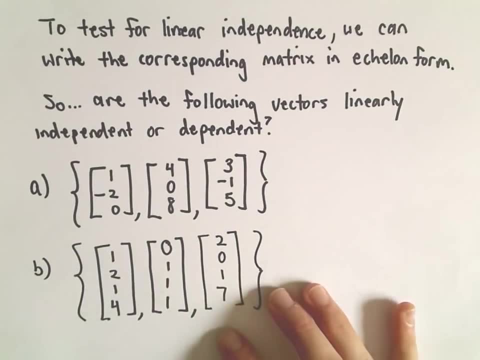 And this is what ties into the notion of the basis for a vector space. But again, we're not there yet. So again, just at this point, think intuitively. Somehow, if you have linearly dependent vectors, those are just linear combinations of other ones. 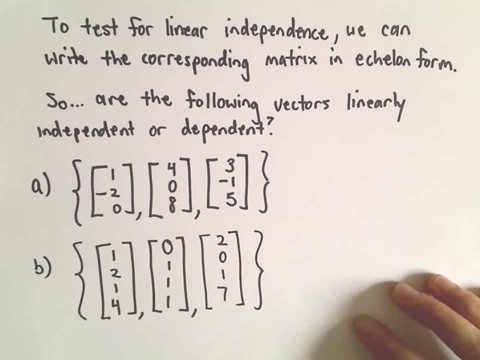 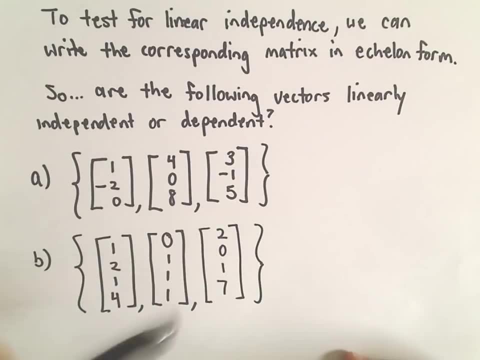 So, in a sense, you can get rid of them and you're not losing any information. That's how I think about it. Okay, so just two questions here. We've got two sets of vectors, two different examples. We'll do these in two different videos. 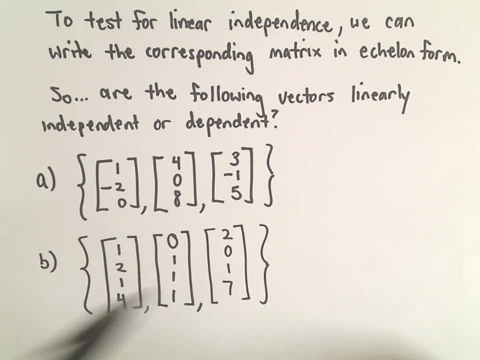 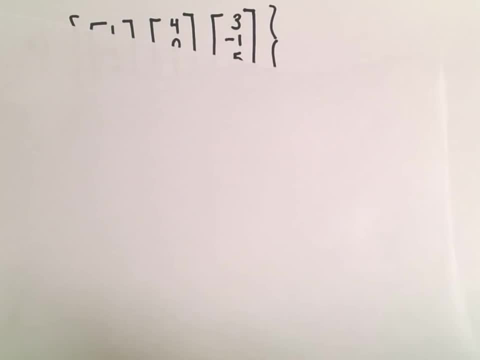 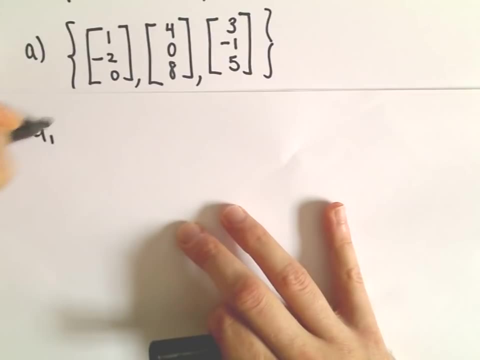 And we're just going to decide if these collection of vectors are linearly independent or dependent. So we'll do part A here first. So again, what we're doing is we're just looking for solutions to the system of equations, or the equation a sub 1 times 2.. 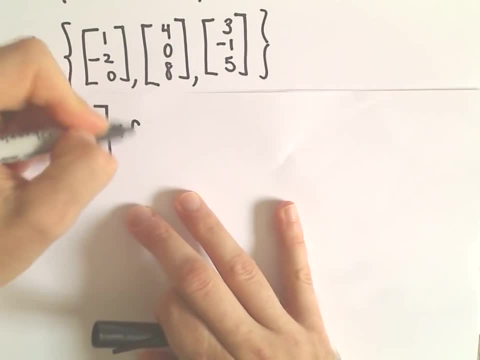 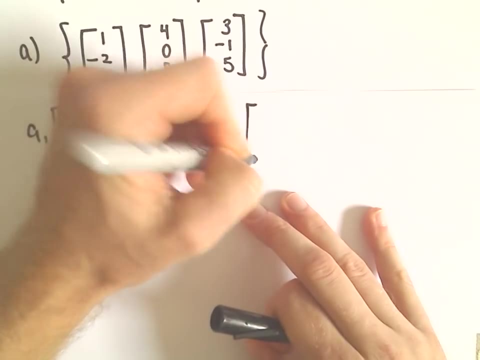 Times 1, negative 2, 0.. Plus a sub 2 times 4, 0, 8.. a sub 3 times 3, negative 1, 5.. And again, we're going to set that equal to the 0 vector. 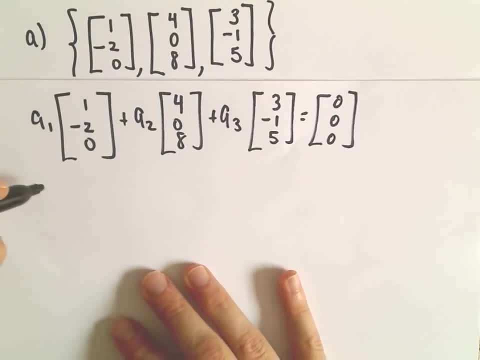 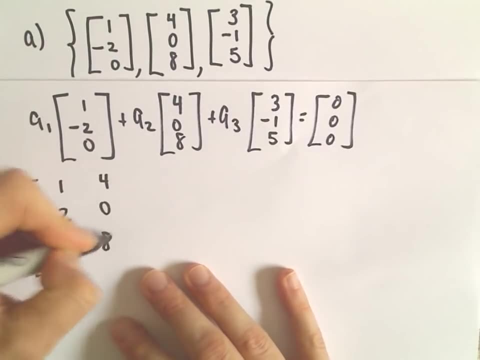 So what I'm going to do is just write this as a matrix and then do some row reduction. So we have 1, negative, 2, 0.. 4, 0, 8.. 3, negative: 1. 5.. 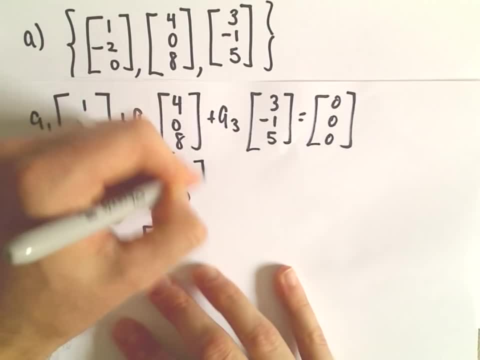 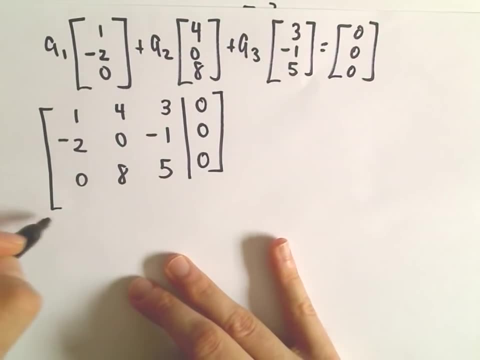 And then 0, 0, 0.. So now again, we're just going to try to put this in our reduced echelon form. So I'm going to do 2 times row 1, add that to row 2 to get my new row 2.. 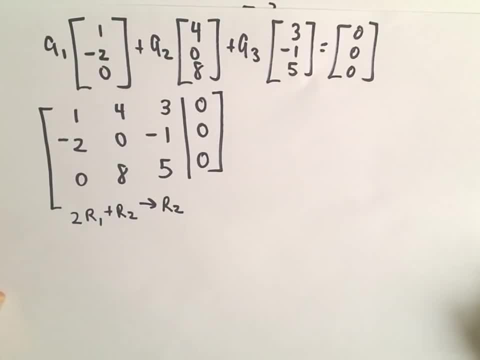 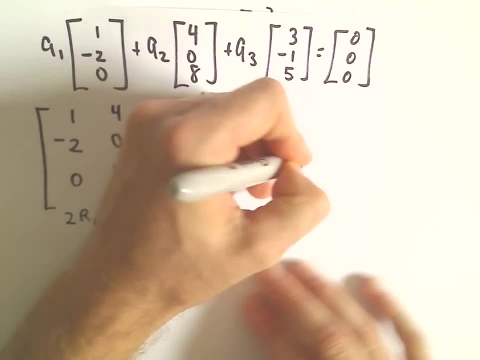 And ultimately, all we're doing is we're just trying to decide if we have trivial or non-trivial solutions. So that's where we're headed. So if we do that, let's see the bottom row we're going to leave alone. 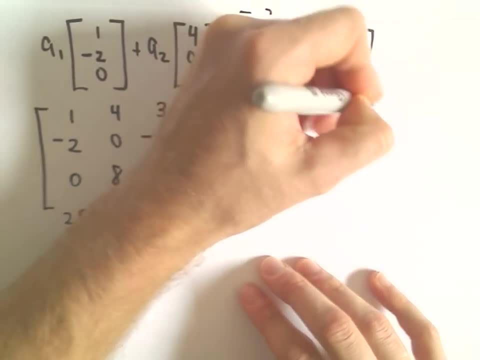 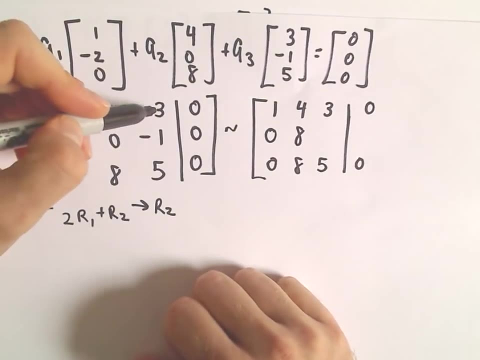 The first row, we're going to leave alone The second row. so 2 times 1 plus negative 2 is 0.. 2 times 4 plus 0 is going to give us 8.. 2 times 3 minus 1 is going to give us 5.. 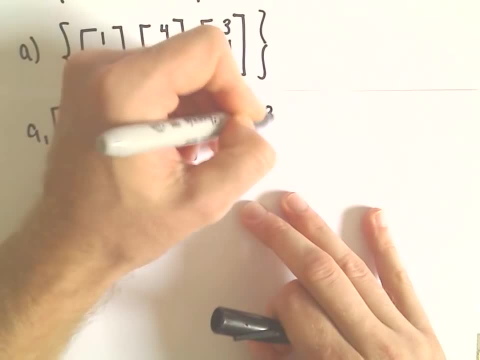 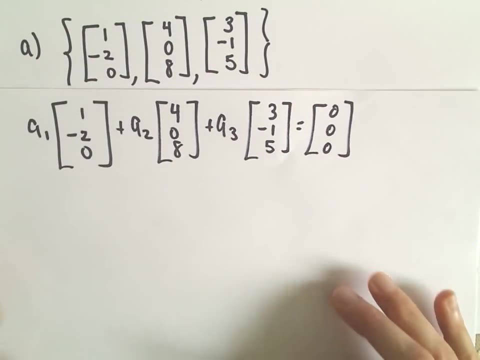 A sub 3 times 3, negative 1, 5.. And again we're going to set that equal to the 0 vector. So what I'm going to do is just write this as a matrix and do some row reduction. 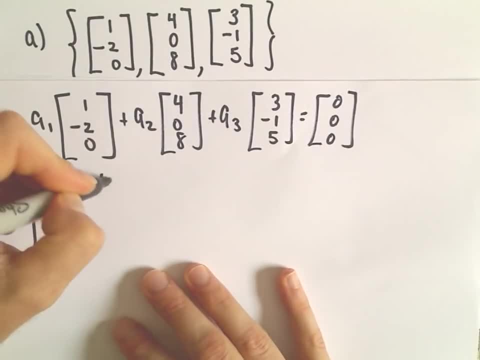 So we have: 1, negative, 2, 0.. 4, 0, 8.. 3, negative, 1, negative 2, 0.. 3, negative, 2, 0.. 3, negative: 0, negative 1.. 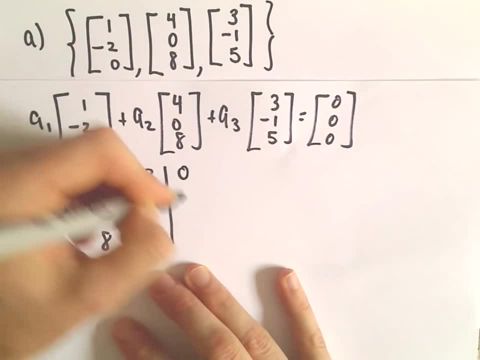 And then again we have A sub 2 times 3, negative 1, 0.. of 1, 5, and then 0, 0, 0.. So now again, we're just going to try to put this in our reduced 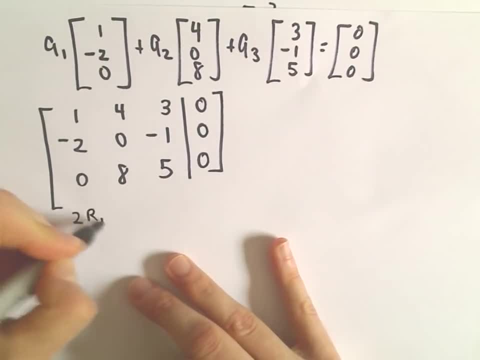 echelon form. So I'm going to do 2 times row 1, add that to row 2 to get my new row 2. And ultimately, all we're doing is we're just trying to decide if we have trivial or non-trivial. 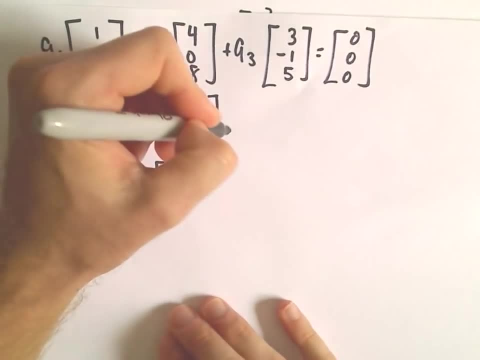 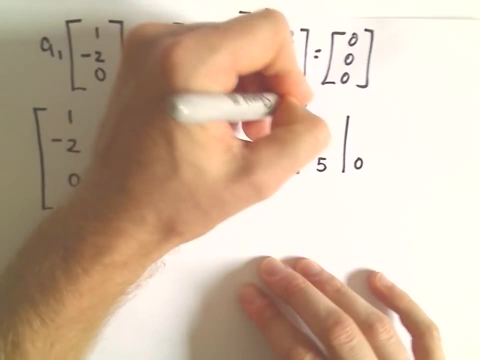 solutions. So that's where we're headed. So if we do that, let's see the bottom row- we're going to leave alone The first row. we're going to leave alone The second row. so 2 times 1 plus. 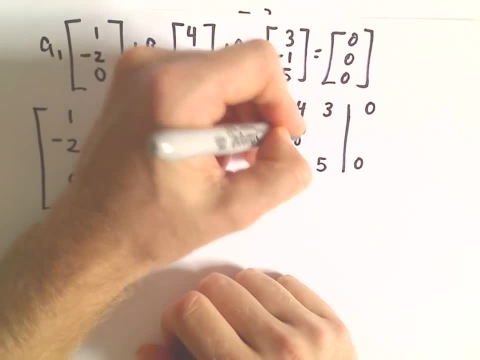 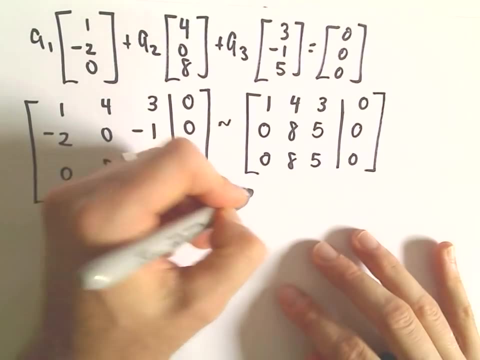 negative 2 is 0.. 2 times 4 plus 0 is going to give us 8.. 2 times 3 minus 1 is going to give us 5.. Oh hey, we've got rows that are exactly the same. I'm going to take negative 1,. 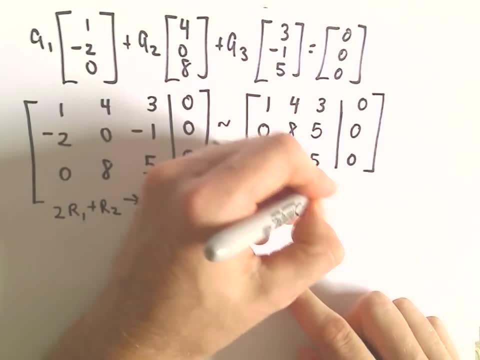 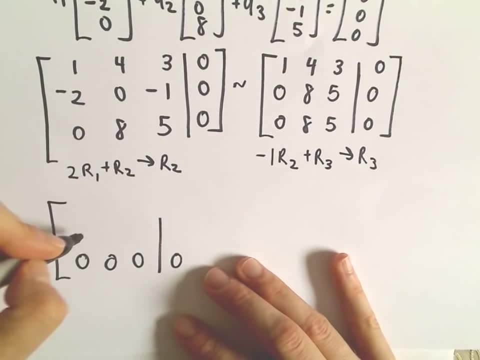 multiply the second row by negative 1, add that to row 3 to get my new row 3.. If we do that, that's just going to make the bottom row all into zeros. Now you may think, hey, automatically you have non-trivial solutions, but we still need to be a little careful. 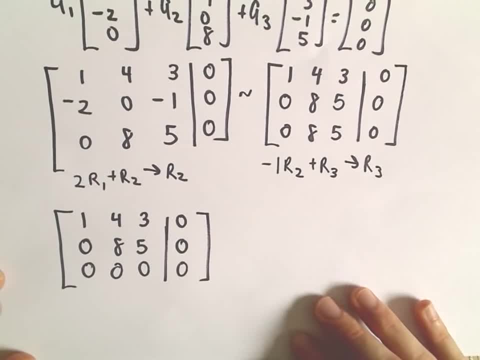 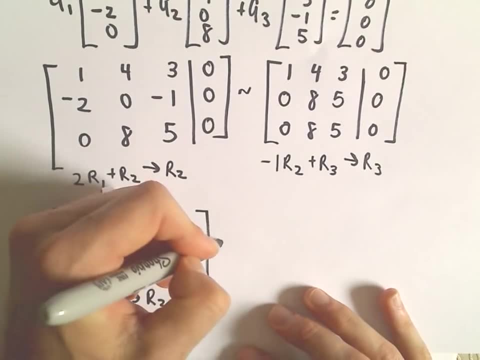 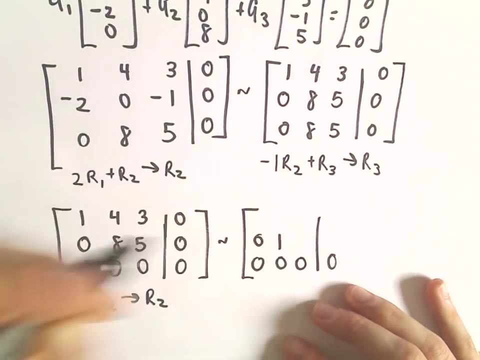 And you'll see this especially in this second example. So I'm going to keep grinding away here. The next thing I'm going to do is just divide the second row by 8.. So if I do that again, we're leaving the third row alone. We'll have 0, 1.. I guess we'll have 5 eighths. 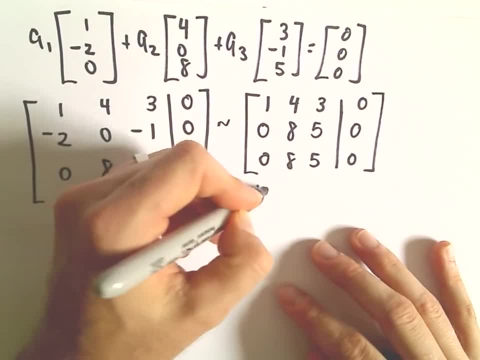 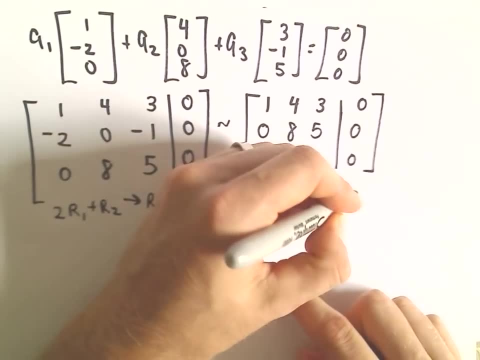 Oh hey, we've got rows that are exactly the same. I'm going to take negative 1, multiply the second row by negative 1, add that to row 3 to get my new row 3.. If we do that, that's just going to make the bottom row all into 0.. 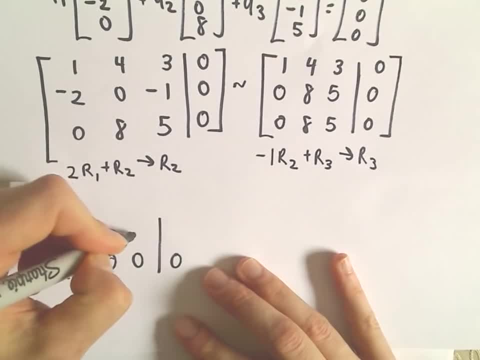 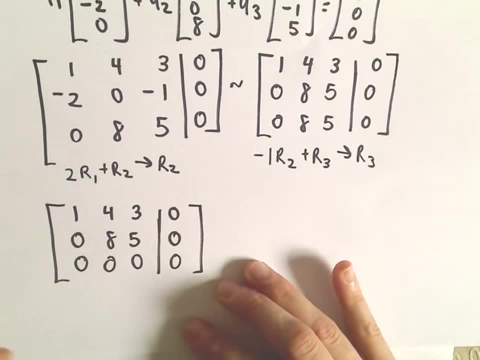 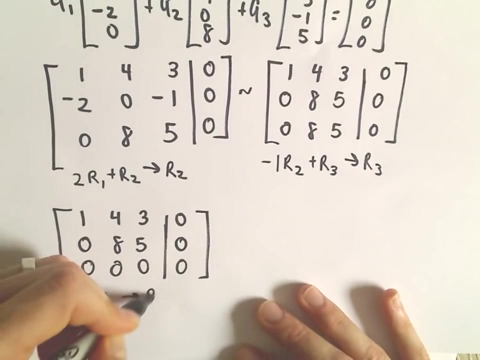 Now you may think, hey, automatically you have non-trivial solutions, but we still need to be a little careful, And you'll see this especially in this second example. So I'm going to keep grinding away here. The next thing I'm going to do is just divide the second row by 8.. 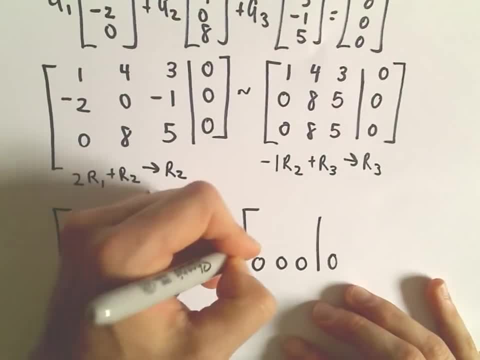 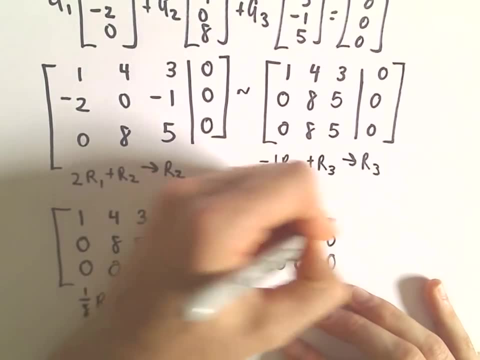 So if I do that, again we're leaving the third row alone. We'll have 0,, 1.. I guess we'll have 5, 8's and then 0. And then we'll have 1.5.. Again, leaving the first row alone. 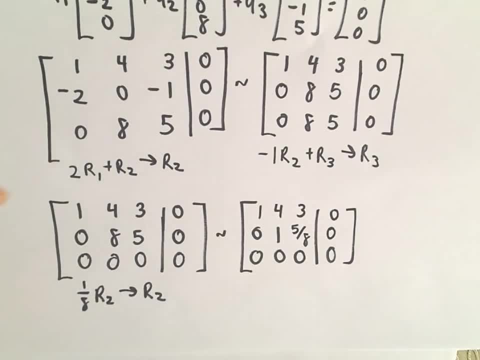 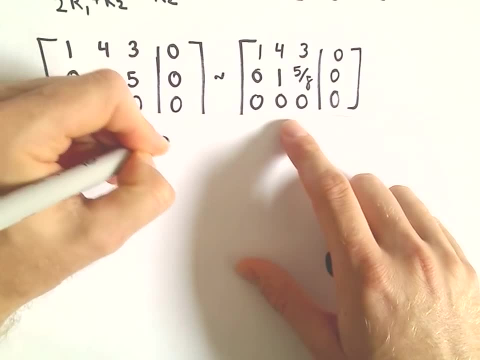 And the last thing I want to do is get a 0 in the first row, second column. So to do that, I'm going to multiply the second row by negative 4 and add that to the first row to get my new first row. 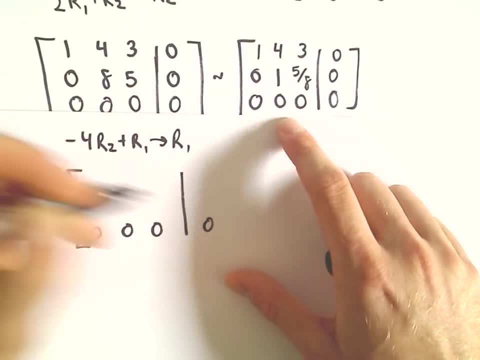 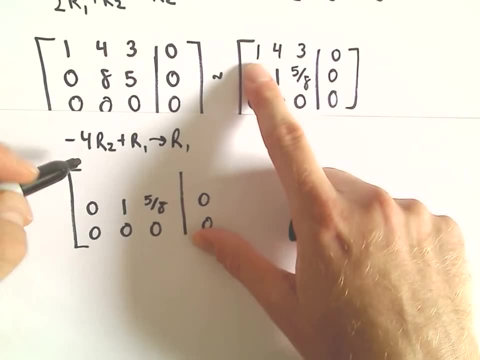 So we have 0, 0, 0 on the bottom, 0, 1, 5, 8's. So let's see, you can check my arithmetic here. So negative 4 times 0 plus 1 is 1.. 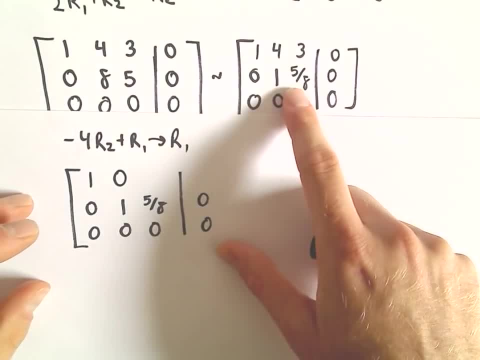 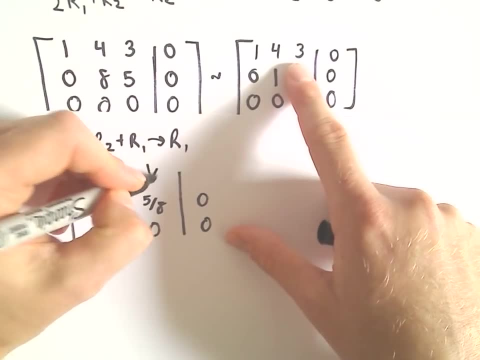 Negative 4 times 1 is negative. 4 plus 4 is 0. Okay, there's the easy part. So I guess negative 4 times 5, 8's that's going to be negative 5 halves. Negative 5 halves plus 3 would leave us with positive 1 half. 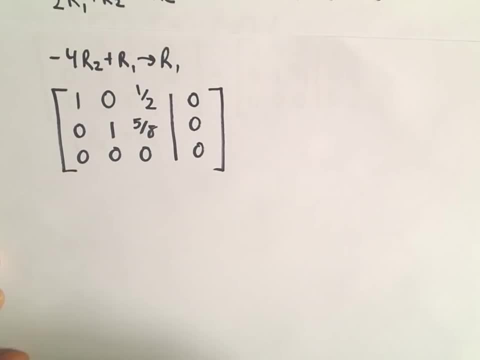 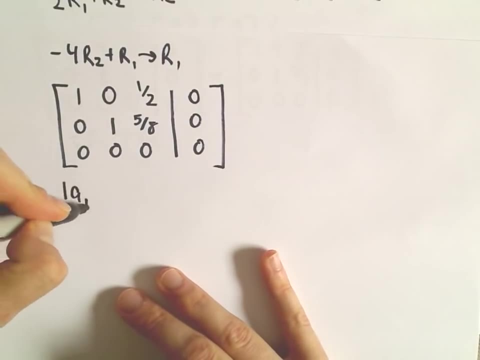 And now to me that looks like a pretty good form. So notice again: you can think about this correspondingly as being the system of equations: 1 a sub 1 plus 1 half of a sub 3 equals 0. So that's going to be: 1 a sub 1 plus 1 half of a sub 3 equals 0. 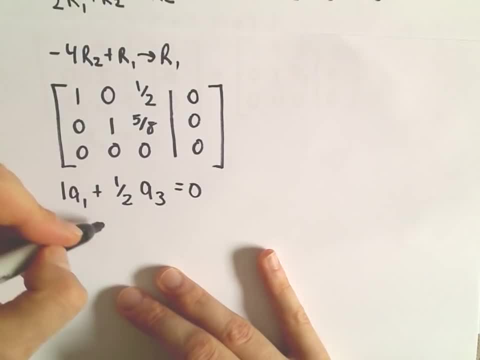 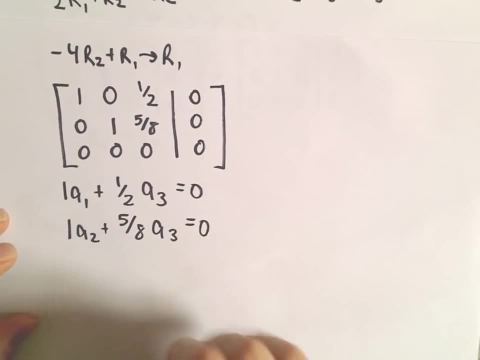 So that's going to be 1 a sub 1 plus 1 half of a sub 3 equals 0.. So that's going to be 1 a sub 1 plus 1 half of a sub 3 equals 0.. We have 0 a 1, we've got 1 a sub 2 plus 5 8's a sub 3 equals 0. 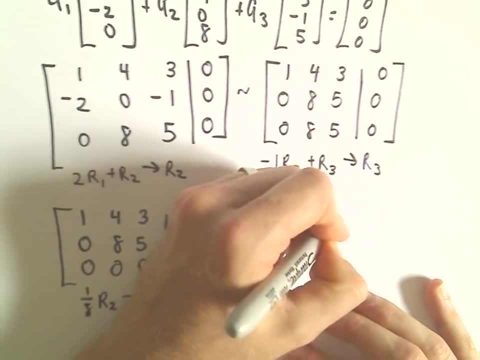 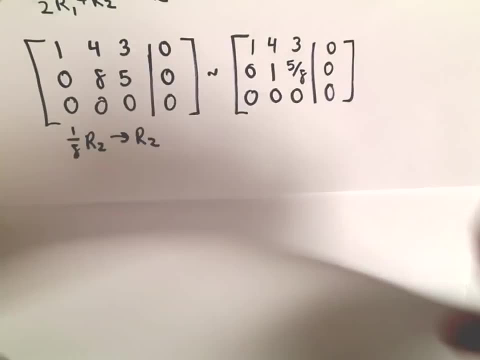 And then 0, again leaving the first row alone. And the last thing I want to do is get a 0 in the first row, second column. So to do that, I'm going to multiply the second row by negative 4 and add that to the first row. 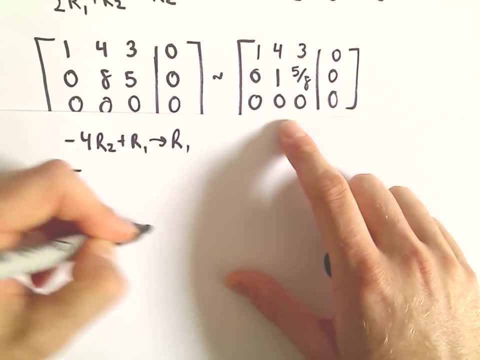 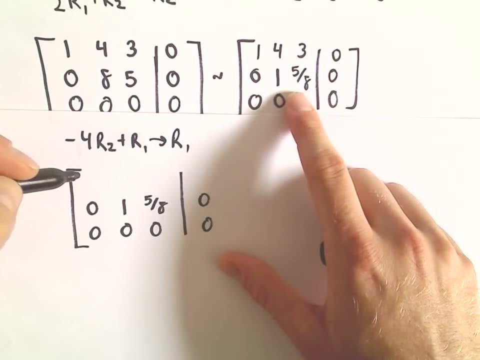 to get my new first row. So we have 0, 0, 0 on the bottom, 0, 1, 5 eighths. So let's see you can check my arithmetic here. So negative 4 times 0 plus 1 is 1.. 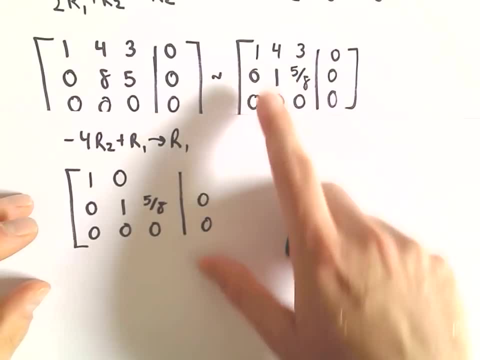 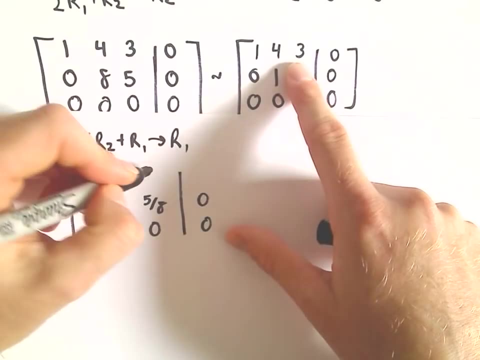 Negative 4 times 1 is negative. 4 plus 4 is 0. Okay, there's the easy part. So I guess negative 4 times 5 eighths that's going to be negative 5 halves. Negative 5 halves plus 3 would leave us with positive 1 half. 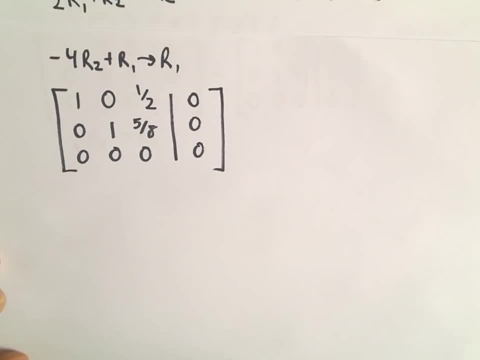 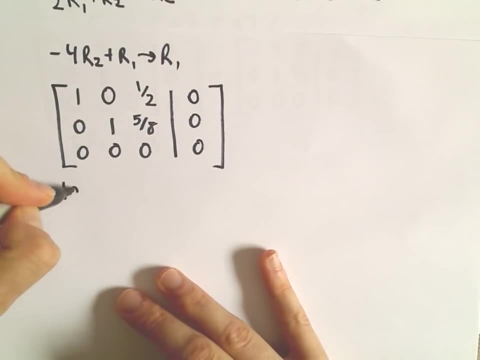 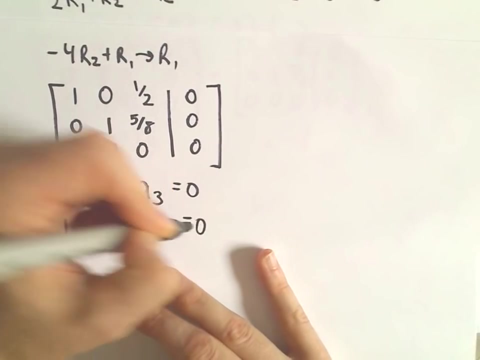 And now to me that looks like a pretty good form. So notice again: you can think about this correspondingly as being the system of equations: 1 a sub 1 plus 1 half of a sub 3 equals 0.. We have 0 a 1.. We've got 1 a sub 2 plus 5 eighths a sub 3 equals 0. 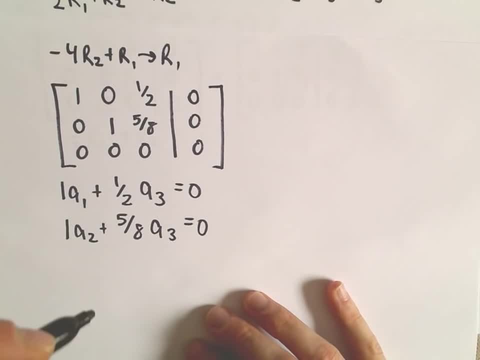 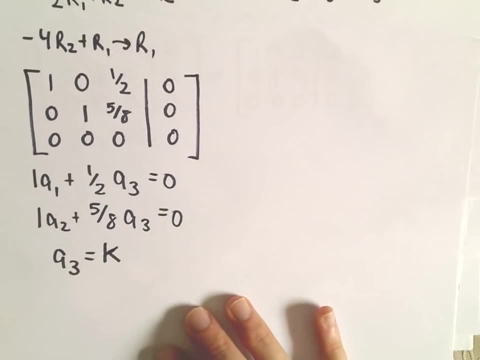 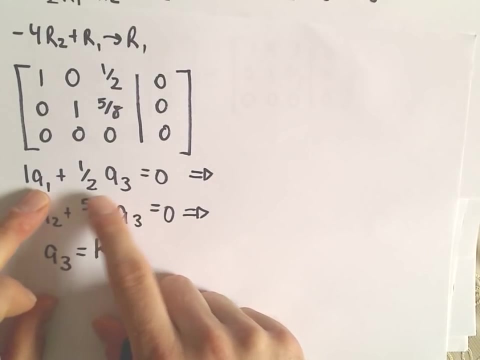 And then our last variable, our last scalar, a sub 3, that's going to be our free variable And we can just set that equal to some number, k. So if we set that equal to k, if we backtrack now, well, if we plug in k, we would get a sub 1 plus 1. half k equals 0. 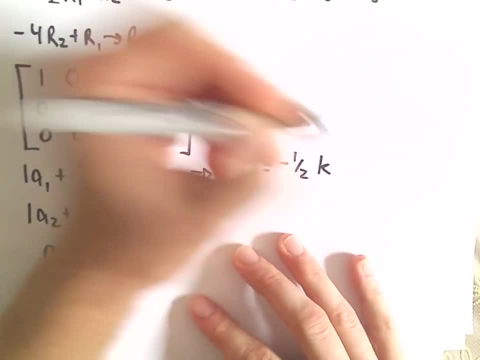 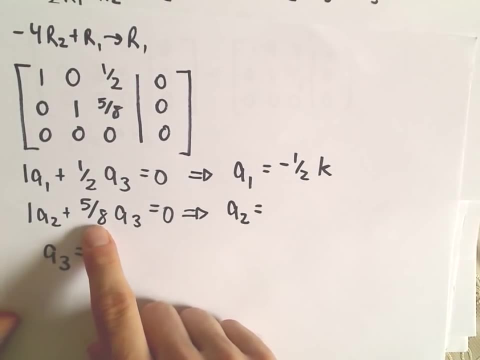 Or we would get a sub 1 equals well negative 1 half times k, And likewise for a sub 2.. If we plug in k, we would have a sub 2 plus 5 eighths times k, equals 0.. 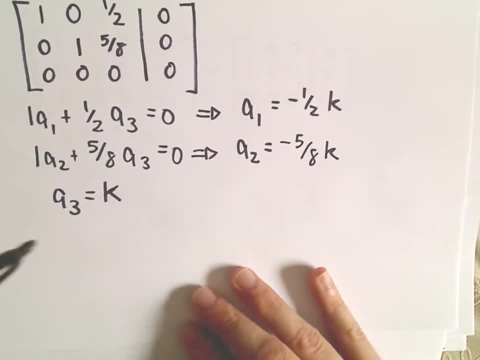 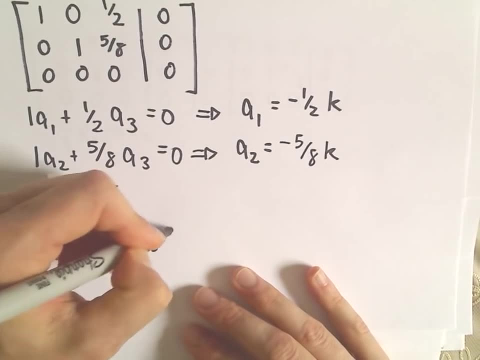 So we would just get negative 5 eighths times k. So it says basically we have non-trivial solutions of the form: Negative 1 half times k, negative 5 eighths times k, And then pick your favorite value for k. 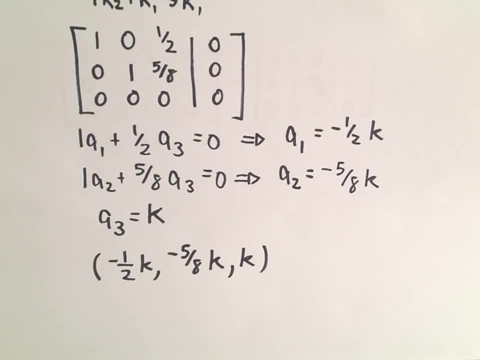 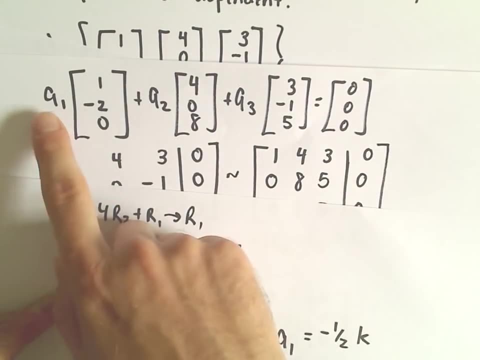 And we'll get lots of different solutions to this original, that original equation that we started with. Okay, so we can figure out different values for a 1, a 2, a 3 by simply picking different values for k. 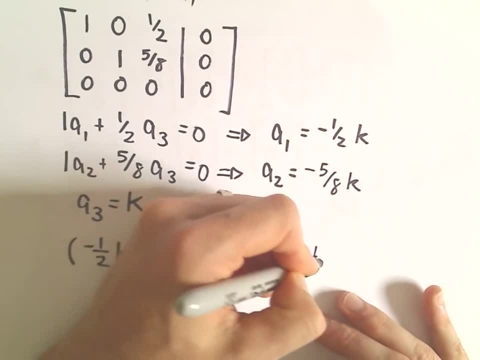 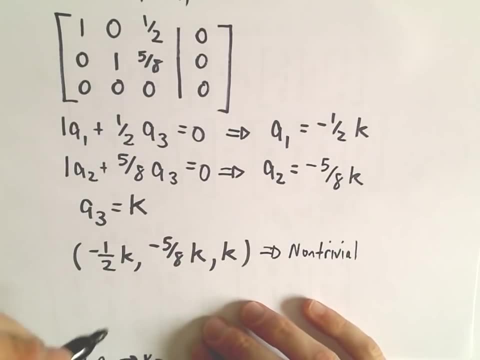 So this tells us we have non-trivial solutions, Which basically means the a sub 1, a sub 2, and a sub 3 value don't have to all equal 0. And that tells us that our set is actually linearly dependent. 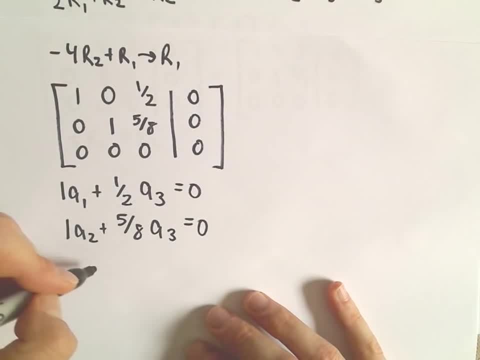 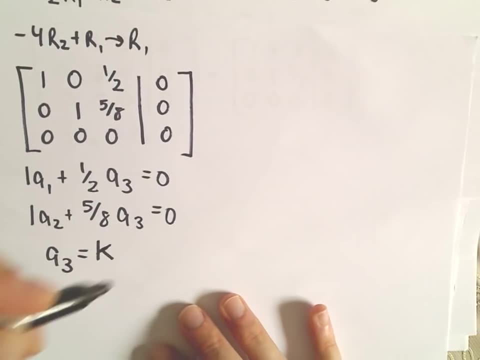 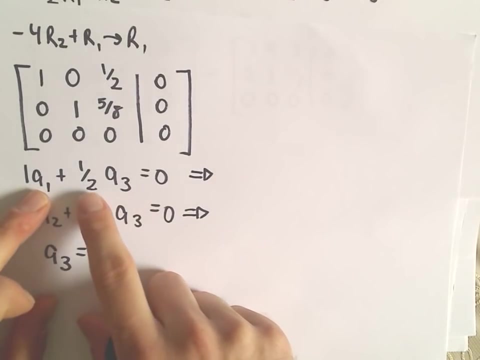 And then our last variable, our last scalar, a sub 3, that's going to be our free variable And we can just set that equal to some number: k. So if we set that equal to k, if we backtrack now, well, if we plug in k, we would get a sub. 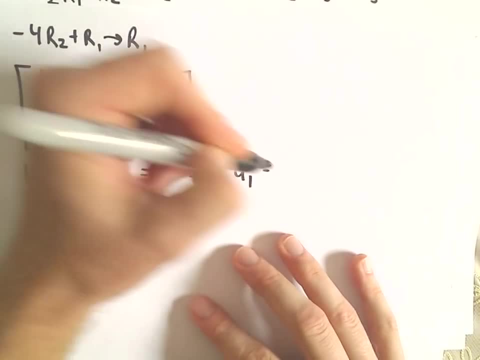 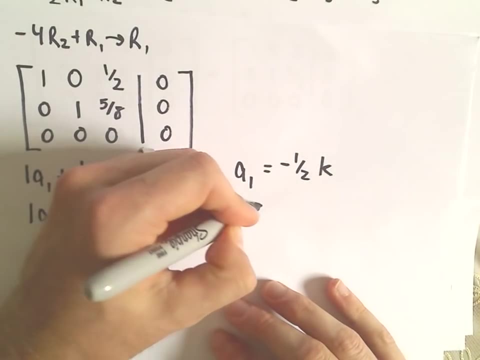 1 plus 1 half k equals 0. Or we would get a sub 1 equals- well negative 1 half times k. And likewise for a sub 2, if we plug in k, we would have a sub 2 plus 5, 8's times k. 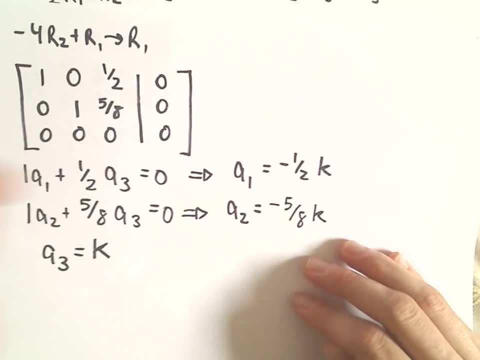 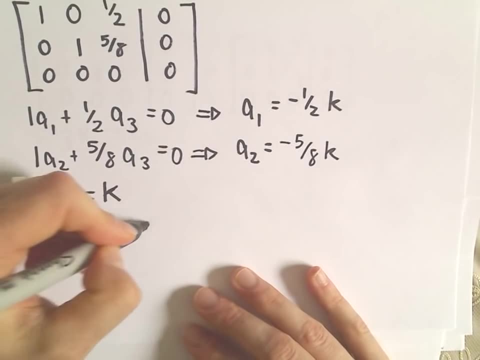 equals 0. So we would just get negative 5, 8's times k. So it says basically we have non-trivial solutions of the form: negative 1 half times k, negative 5, 8's times k, And then pick your favorite value for k. 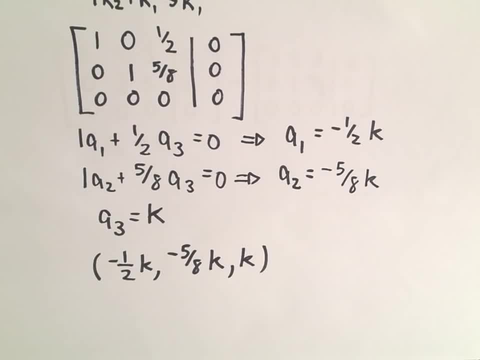 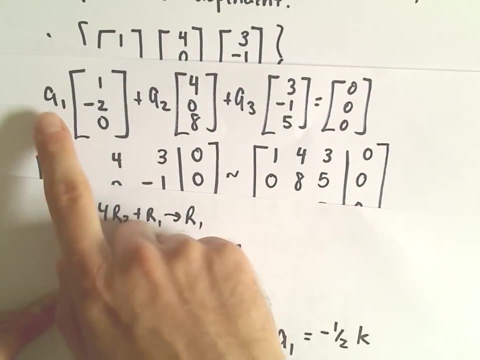 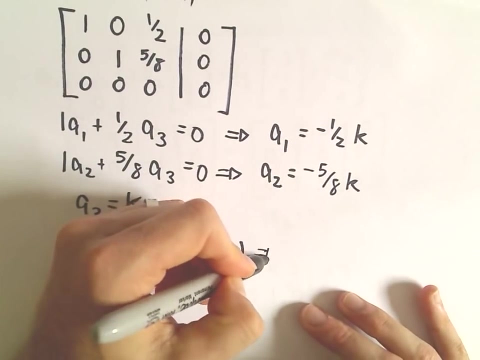 And we'll get lots of different solutions, solutions to this original, that original equation that we started with. Okay, so we can figure out different values for A1, A2, A3 by simply picking different values for K. So this tells us we have non-trivial solutions, which basically means the A sub. 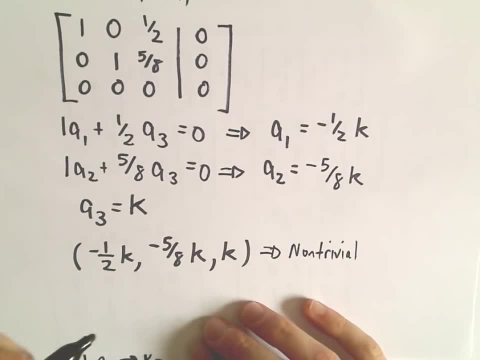 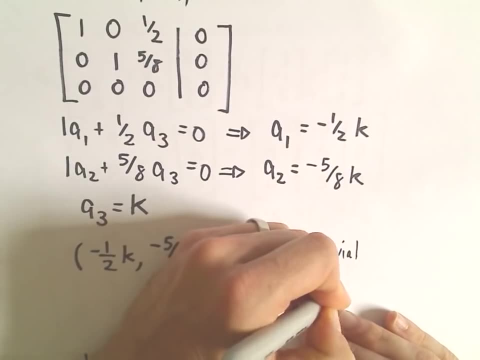 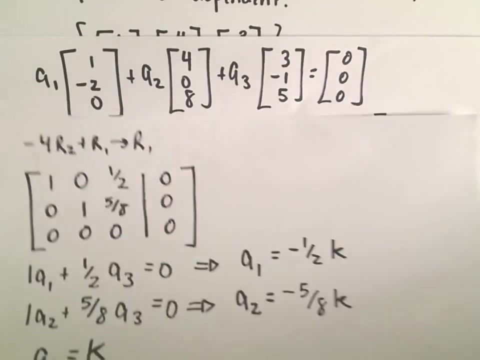 1,, A sub 2, and A sub 3 value don't have to all equal 0, and that tells us that our set is actually linearly dependent. So we could have taken one of those vectors out. in this case is what's happening? 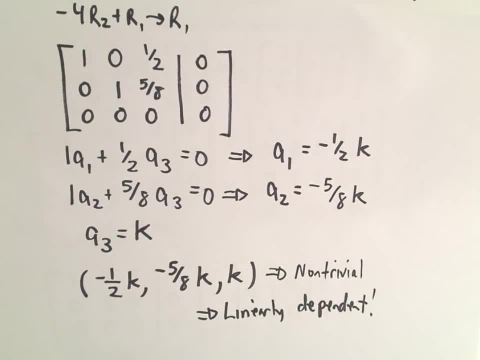 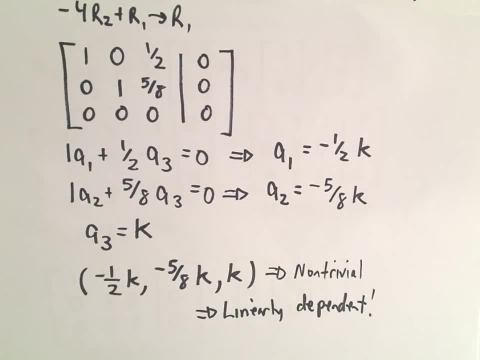 So that's all there is to it. You're just doing a little row reduction. So I'm going to do the other example as well. You'll see the same thing happens. We'll get a row of zeros, but it still turns out that in this case- well, we actually end. 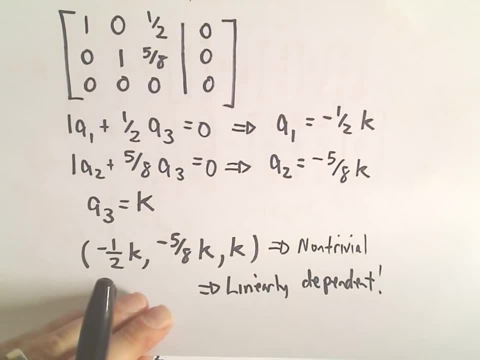 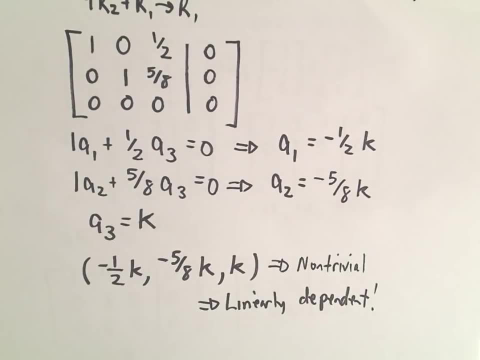 up with a linearly independent set in part B. But if you want to definitely take a look at that, We'll step through it and then we'll tie this notion together- you know, linearly independence- and this notion of a span to create what's called a basis for a vector. space.